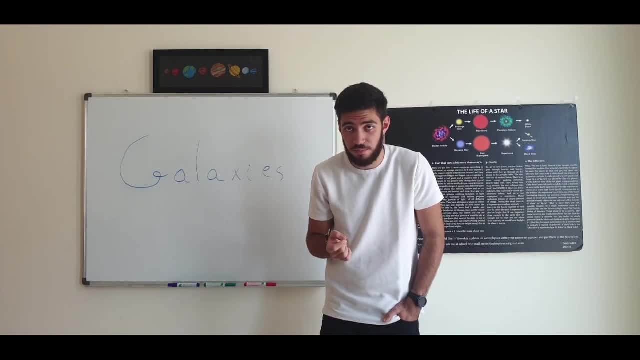 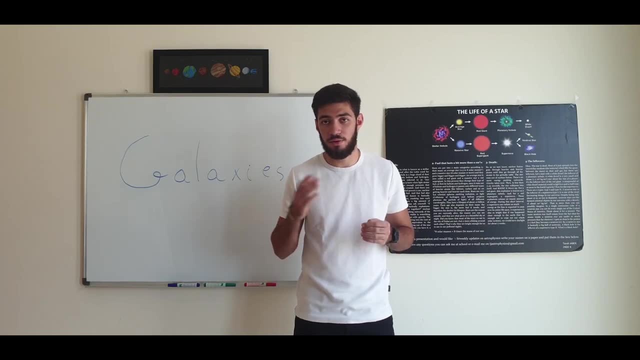 ideas about their origin and how they evolve. Now, obviously, a human lifespan is not long enough, not nearly long enough to watch a galaxy form and grow. But using very, very big telescopes and supercomputers, astronomers can look deep into space, which, because light needs time to get to us, is equivalent to: 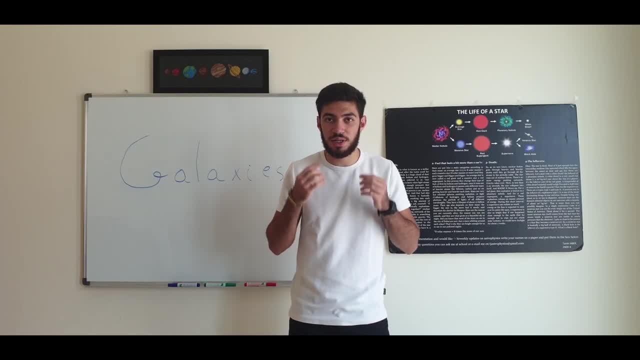 looking back in time And by doing that, astronomers can observe different stages of galactic evolution and have an idea of how they form and evolve. You can think of it this way: if you point a camera at a person, for 10 minutes, you're. 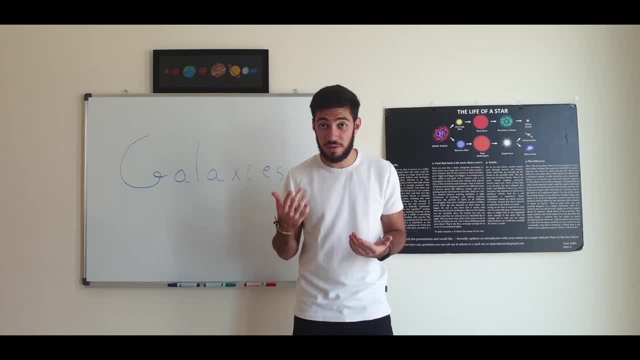 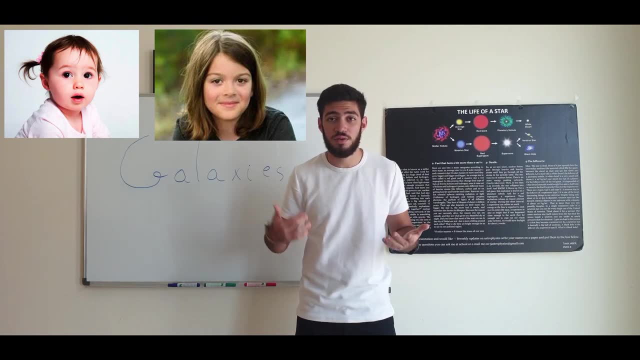 not going to have a single idea about human evolution, But if you look at different people around the world- a person that's two years old, another that's 10,, one that's 15,, 20,, 30,, 40,, 80, you can have an idea about how. humans evolve. Astronomers did exactly that and found that galaxies formed fairly soon in the universe, so around 300,000 years after the Big Bang, when the whole universe was filled with mainly hydrogen and helium, with some areas denser than others. Gravity caused these dense areas to collapse into clumps or clouds of gas, start nuclear fusion and start the first generation of stars. Gravity would then even cause multiple clouds to themselves collapse into each other, forming bigger clouds, accumulating eventually to becoming rotating disks. So, after forming 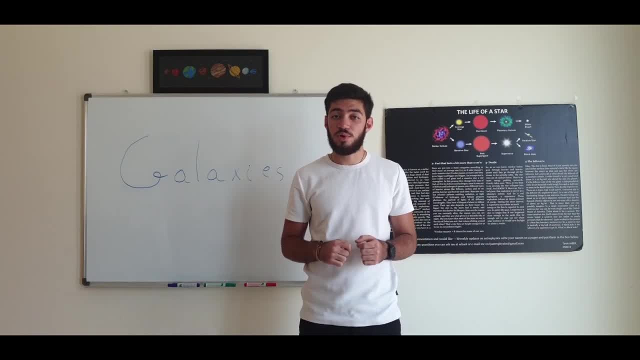 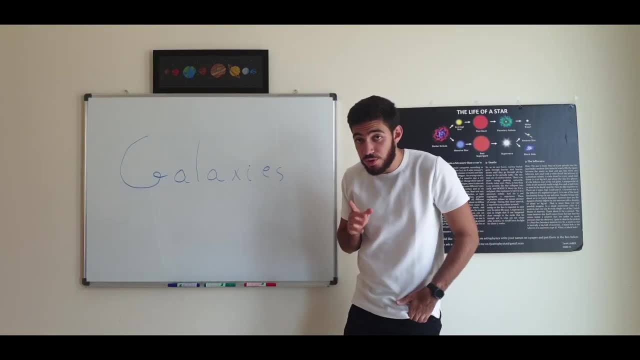 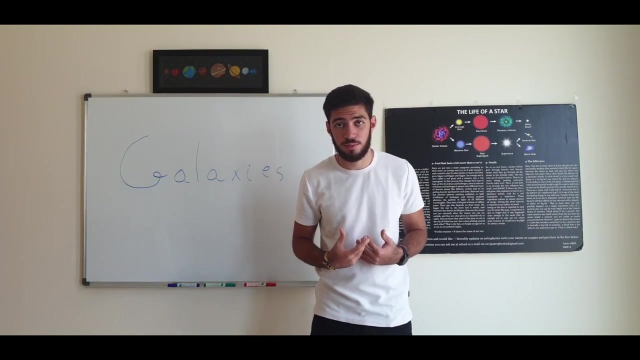 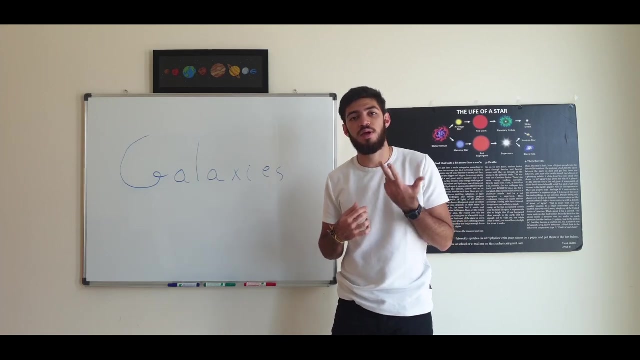 galaxies evolved to have more stories and more defined shapes, as we can see in this video. Astronomers also discovered that in the center of most large galaxies exists a supermassive black hole. Now moving on to the different types of galaxies, Astronomers classify galaxies in three main. 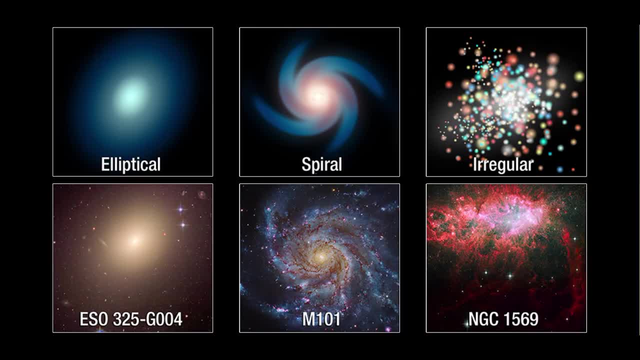 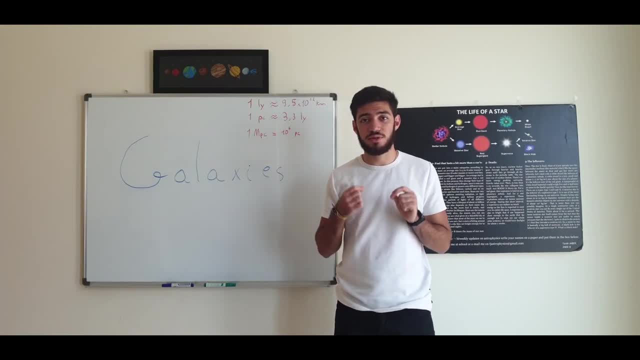 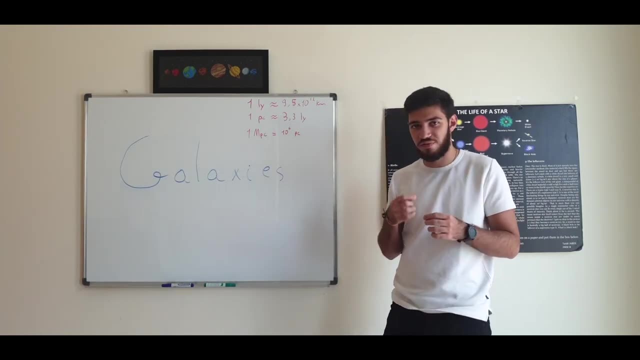 categories: Irregular, elliptical and spiral galaxies. Now, before we dive into the details of each of the categories, we need to define the units we're going to be using to describe these big distances. The first one is the light-year, which is equivalent to around 9.5 times 10 to the power. 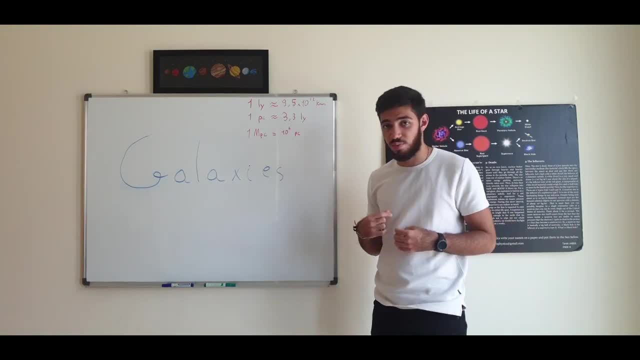 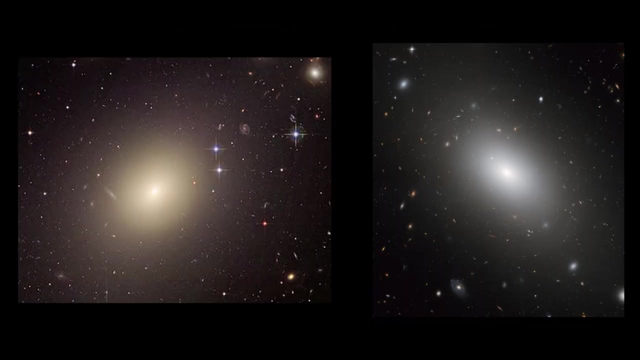 of 12 kilometers. The other one is the parsec, which is equivalent to approximately 3.3 light-years, and the final one is the megaparsec, which is a million parsecs. So let's start with elliptical galaxies. Here are some pictures. Elliptical galaxies vary. 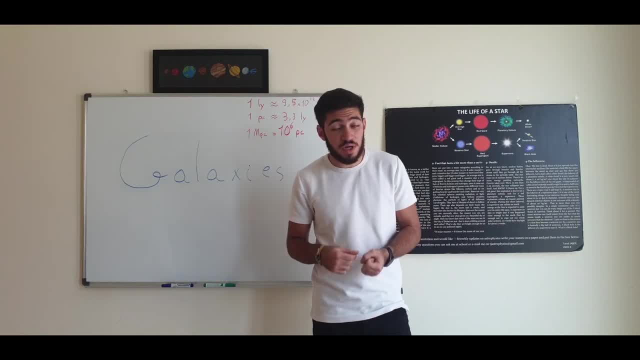 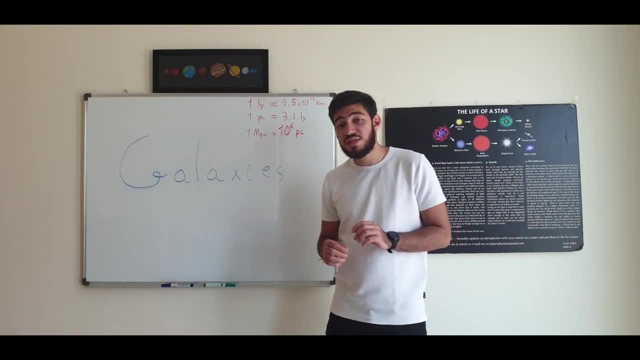 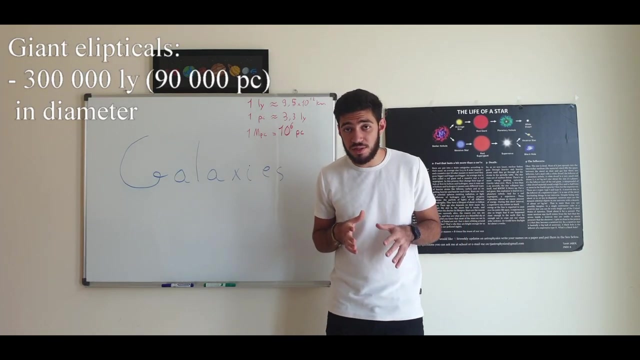 from nearly circular to very elongated. These types of galaxies are not as active anymore, meaning that they're not forming as many stars as they used to. The biggest elliptical galaxies are called well giant ellipticals, and they measure about 300,000 light-years or about 90,000 parsecs in diameter. The smaller and more 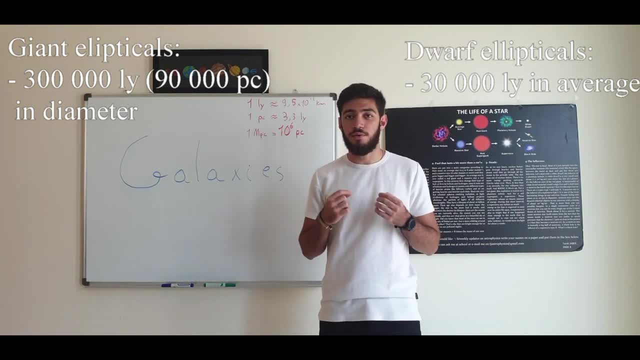 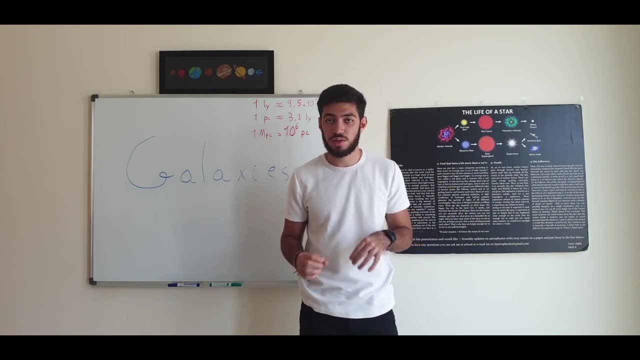 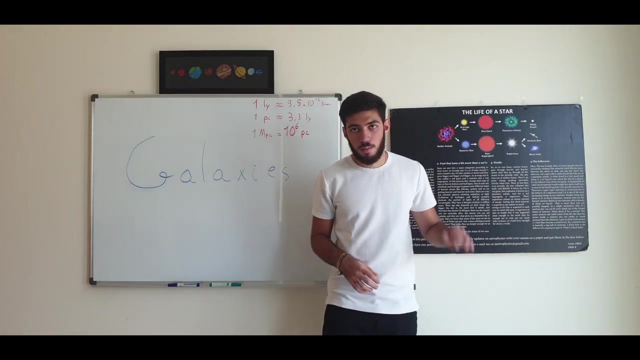 common ones are called dwarf ellipticals and only have a diameter of a few thousand light-years. Now we move on to spiral galaxies like our Milky Way, And here are some examples of spiral galaxies. Here are some pictures of some others. Spiral galaxies fall into two main subcategories: barred spiral galaxies and normal spiral galaxies. Both these subcategories are pretty similar. The only difference is that barred spiral galaxies have a bar going through the center of the galaxy, while normal spiral galaxies don't. The third and last main category of galaxies are irregular galaxies. These galaxies have very little dust and are not disc-shaped nor elliptical. but as 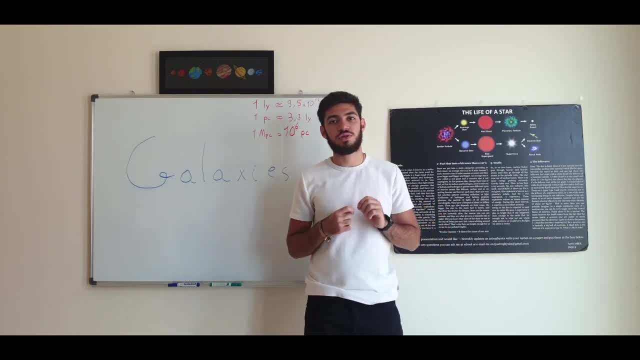 their name states, irregular, They don't really have a certain shape or size. Now, most of the observed irregular galaxies were observed deep into the universe, far from us, which, as we said earlier, is equivalent to looking back entirely. Now this tells us. 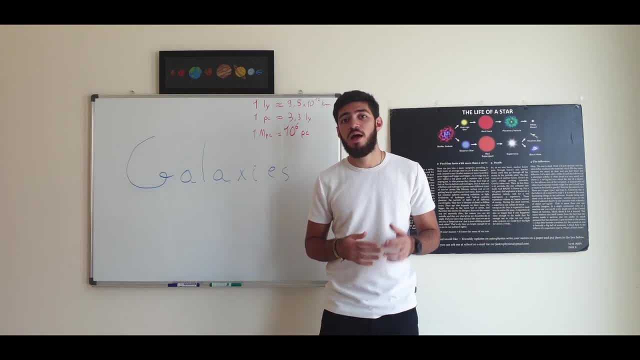 that these types of galaxies were abundant in the early Universe and appeared before elliptical and spiral galaxies did. So. those are the three main categories of galaxies: spiral galaxies, elliptical galaxies and irregular galaxies. Galaxies, despite being very, very far from each other, still form groups called clusters. 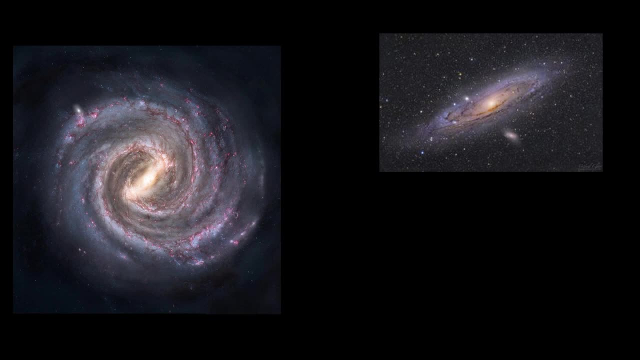 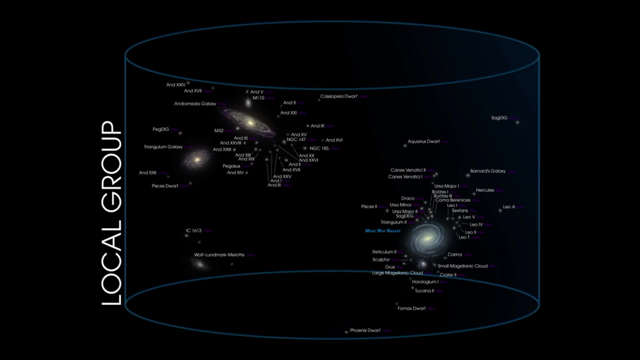 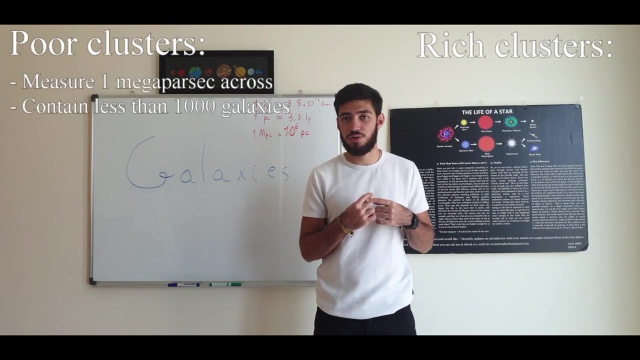 For example, our galaxy, the Milky Way and the Andromeda Galaxy, the Large Magellanic cloud and the small Magellanic cloud are all part of a cluster called the local group. Now there are two types of clusters: poor clusters and rich clusters. Poor clusters measure only. 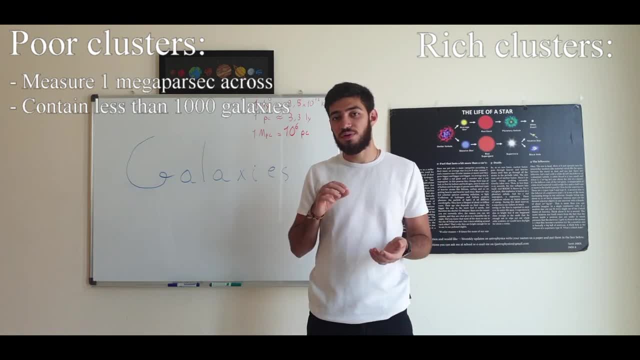 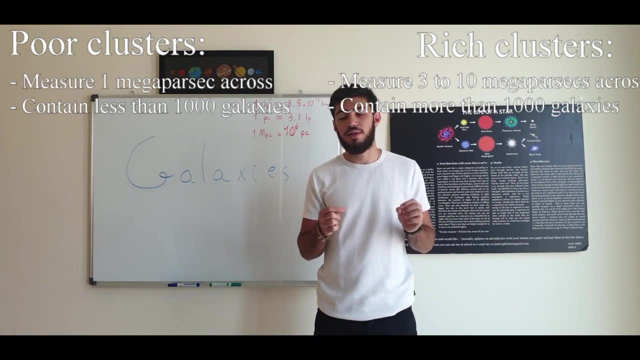 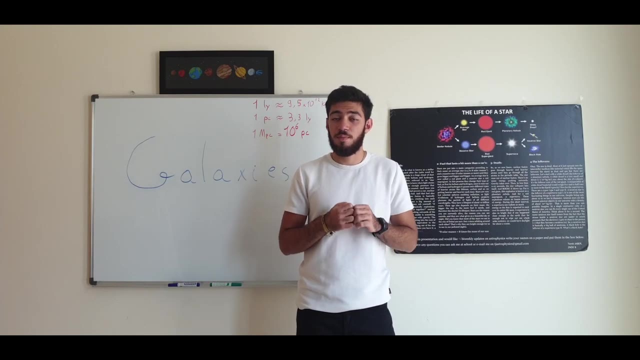 about one megaparsec across and have about a thousand galaxies, while rich clusters measure three to ten megaparsecs across and have thousands and thousands of galaxies in them. An example of a rich cluster is the Virgo cluster, measuring about 3 megaparsecs across, having over 2000.